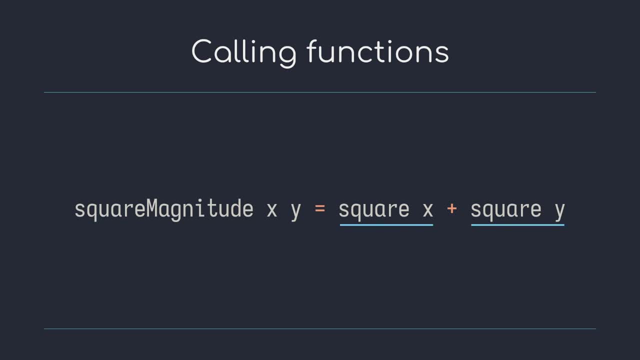 once again use spaces to separate the arguments and function name from each other. This doesn't mean we never need to use parentheses, though. If the argument you want to pass is an expression containing spaces, you need to enclose it in parentheses like this: 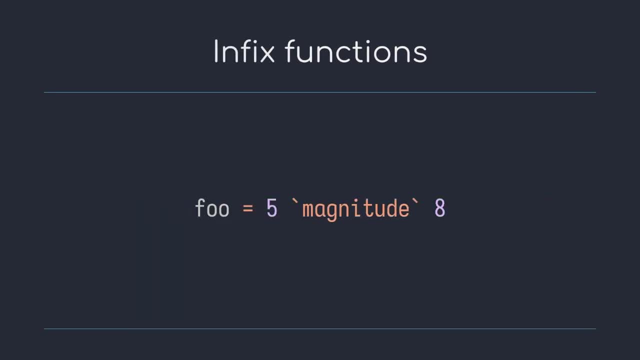 Haskell actually allows you to call every binary function as an infix function by surrounding the function name with backticks. This can be useful for reducing the amount of parentheses in some cases, but it can also make your code a lot less readable, so use it carefully. 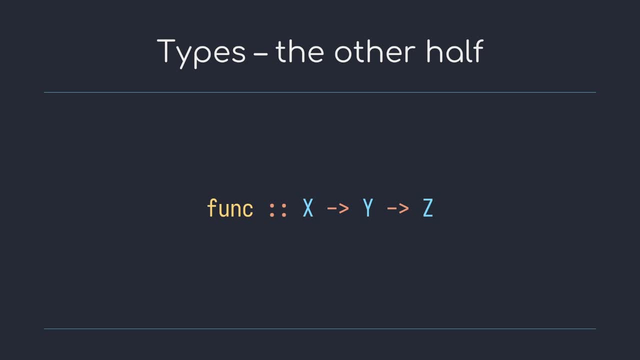 Another key part of the Haskell language is the type system. Up until now, I only showed you half of the code that you should be writing when creating functions. Every function should be supplied with a type which is written like this: This would describe a function that takes two arguments of type x and y and produces 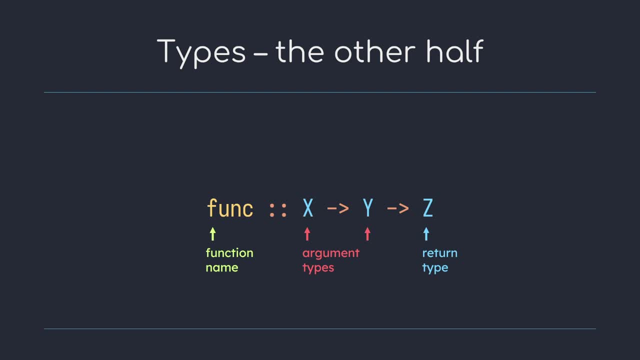 a result of type z. Notice how the return type of the function is not denoted separately from the argument types. This again has to do with currying. Don't worry, just a couple more things and I'll explain what it is promise. 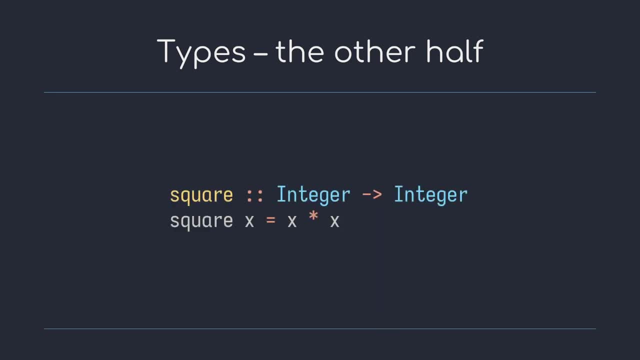 For example, the type of our square function we made earlier would look like this: Some functions work for more than one discrete type, like functions that operate on lists or numbers. In order to deal with this, Haskell allows you to use type variables. These will assume: 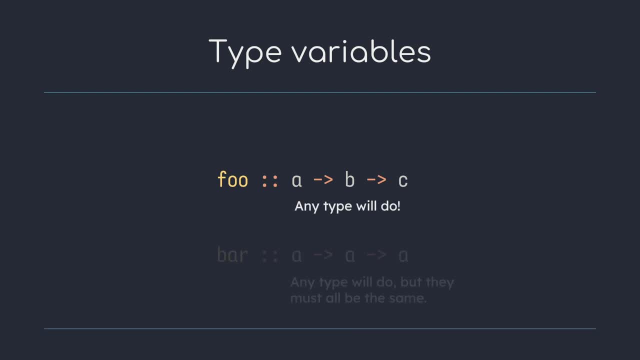 any type you provide them. If two type variables have the same name, however, they must always be the same type. A good example of this is the hat function provided by the standard library. It takes a list of some type a and returns the first element of that list, which of course has 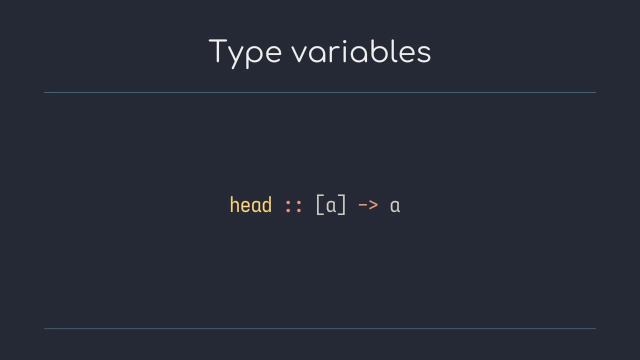 type a as well. This function can now be used for lists of all types, not just one specific one. Let's use this to generalize our square function, right. There is one problem, however, When we try to change the integer types to type variables. 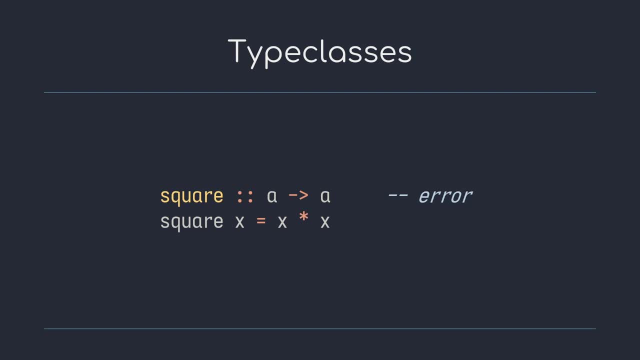 we get a compiler error, This is because we are using the multiply operation, which only works for numbers. But right now we are specifying our function accepts all types, not just numbers. We need a way to restrict the type a can assume, so it only accepts numbers. 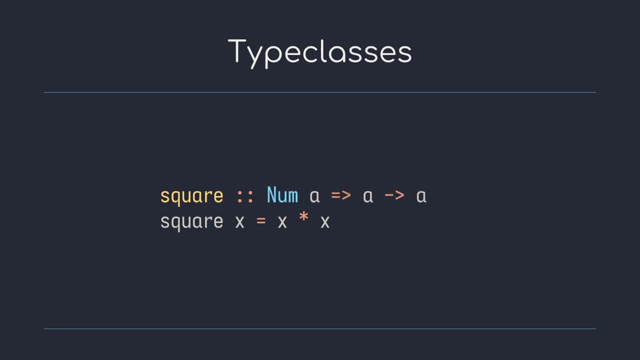 This is done with the numType class. A type class is a description of what functionality a type must implement in order to derive from it. It is a lot like an interface in that regard. This type would read: function square has type a to a, where type a is an instance. 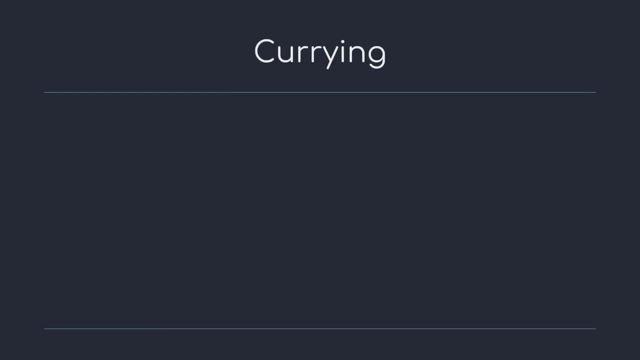 of num. So what is this currying thing I mentioned earlier? I'll have to disappoint you that it is in fact not related to curry, but it is still very neat. Basically, currying allows us to leave out some of the arguments in a function until later. How does this work? Well, 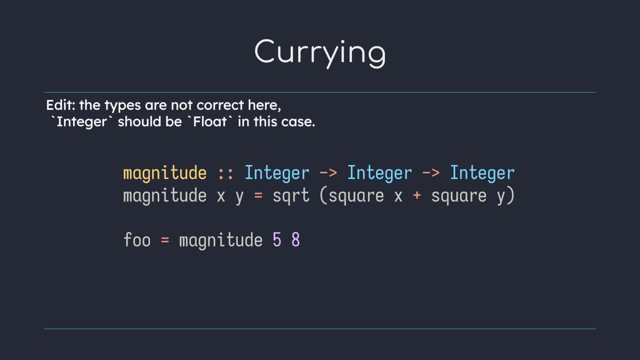 let's grab our magnitude function from earlier. In this case, full would just be our return value. So what happens when we don't provide the second argument 8?? Interestingly, we don't get a compiler error. This is because full has now become a function and this is 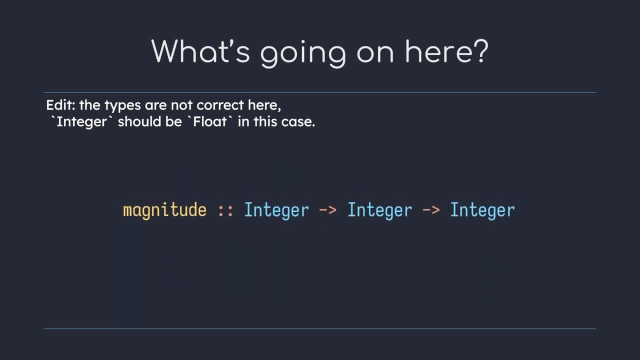 its type. If you look at the type of magnitude again, it's like we have shaved off the first argument and are now left with integer to integer. If we then provide another argument, will be left with a function that takes zero arguments, which is just the integer value. 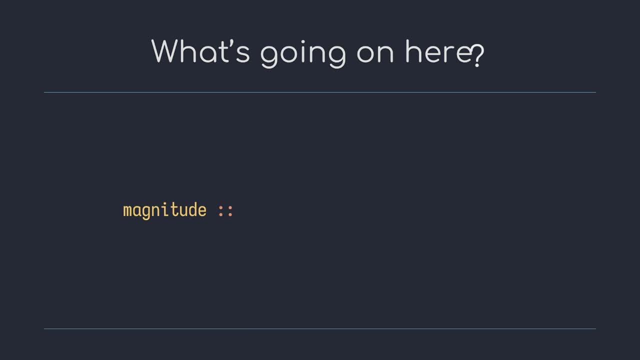 This is a very useful tool in Haskell and makes modifying and combining functions a lot simpler. So what if I want to create a branch in my code? Where are my if-else statements? Haskell has three main methods for branching your code. The first one is if-then-else blocks. An if-then-else block is more like a 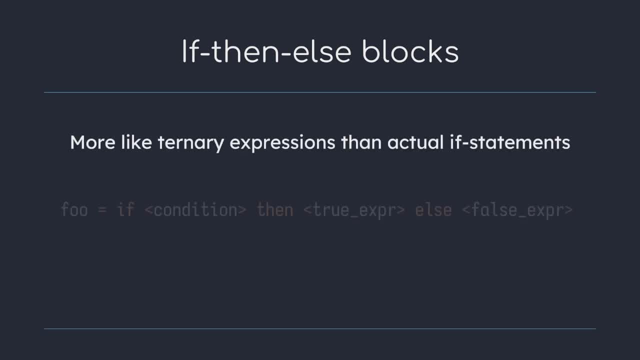 ternary expression than an actual if statement. It takes a condition and evaluates through the first expression when it is true and the second expression when it is false. Haskell has no else-if blocks, however, so when you need to check for multiple conditions, you have to use nested if statements or use one of the other methods for branching. 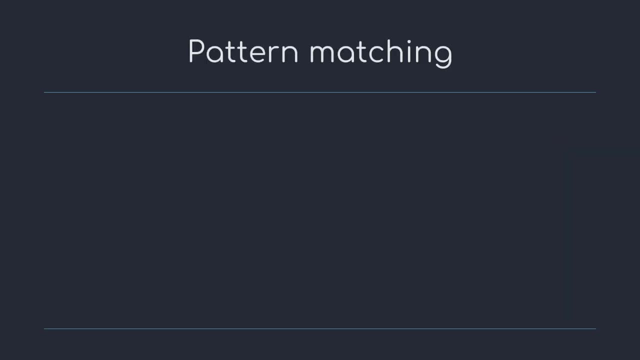 Pattern matching is a bit of syntactic sugar that allows us to control the flow of the function by matching over the arguments. For example, a function that returns one when the number is zero but returns the number itself otherwise can be written like this: Haskell will match the provided arguments against every pattern, starting from the top.